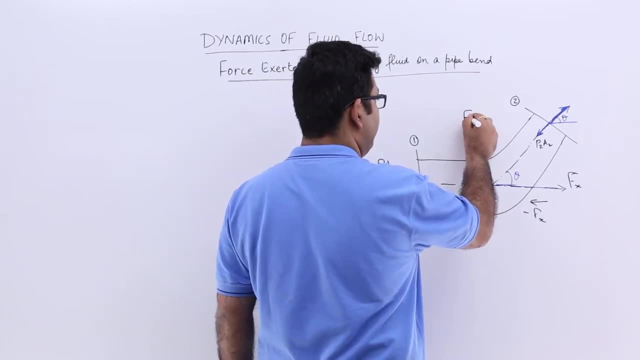 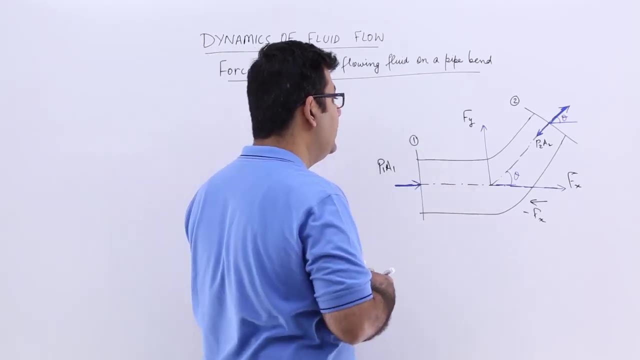 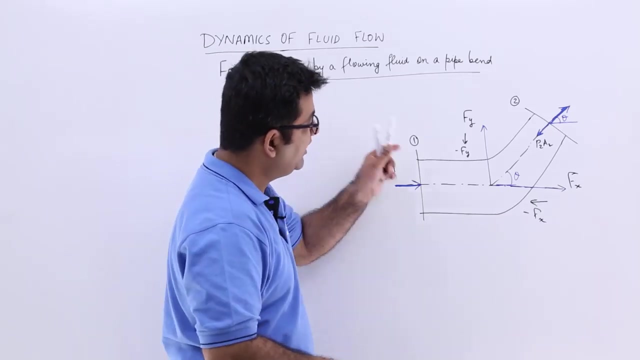 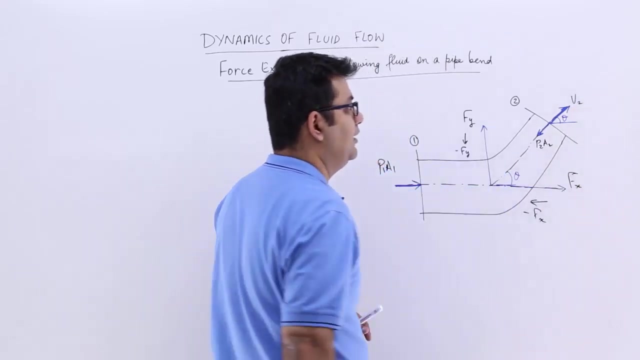 Okay, Similarly, you will have some vertical component also, That is, the force exerted by the fluid on the bend, and you will have an opposite force minus Fy, which is the force exerted by the bend on the fluid. And let us say that this is the velocity at exit- V2- and you will have a velocity at inlet as V1. 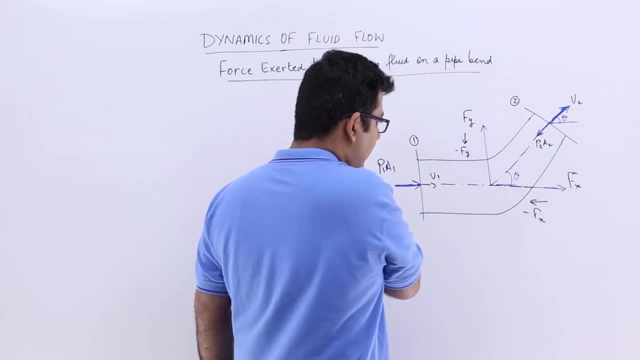 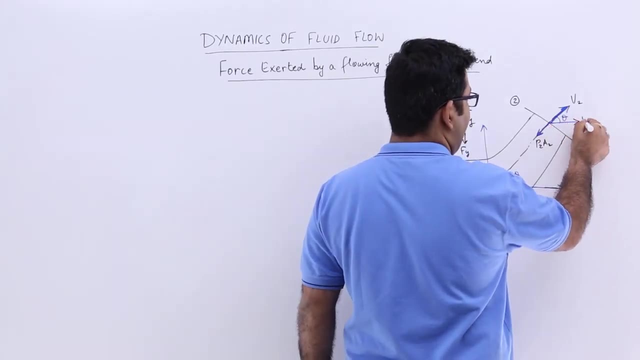 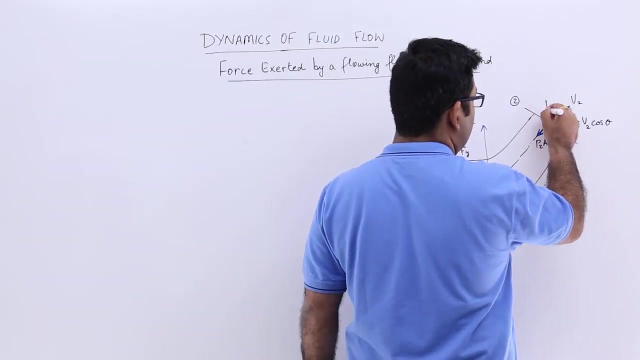 Okay, So the direction of exit and the direction of inlet has an angle of theta in between them. So if this is V2, this will have a horizontal component, which is V2 cos theta, And it is going to have a vertical component also, which is V2 sin theta. 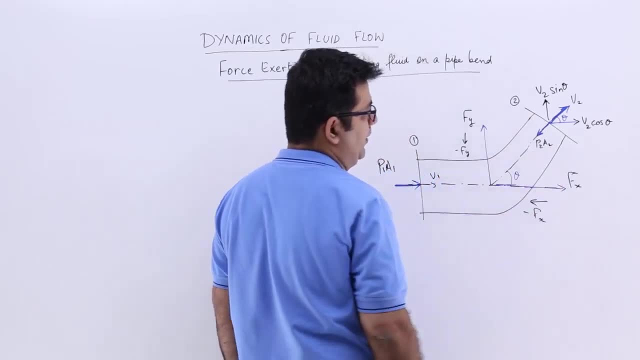 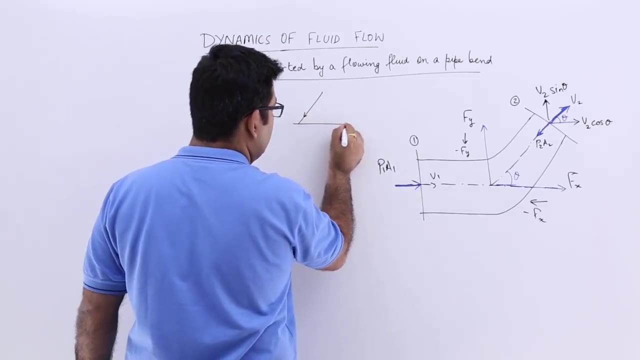 Alright, So accordingly, I can also split up P2 A2 into its two components, So you will have: This is P2 A2.. Okay, And you will have two components of this. So this is theta P2 A2.. 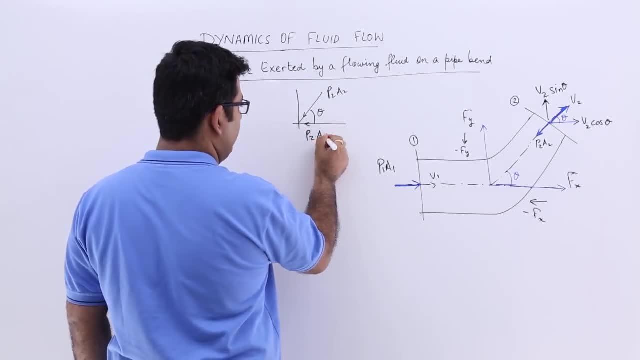 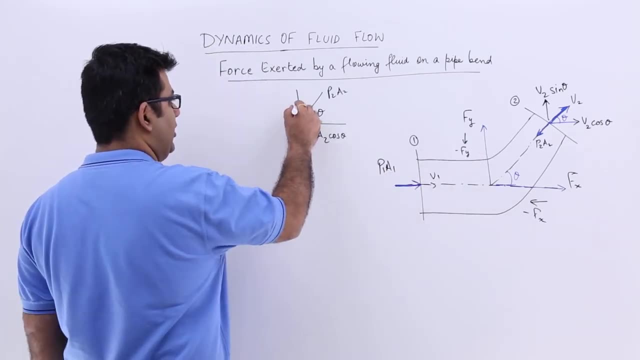 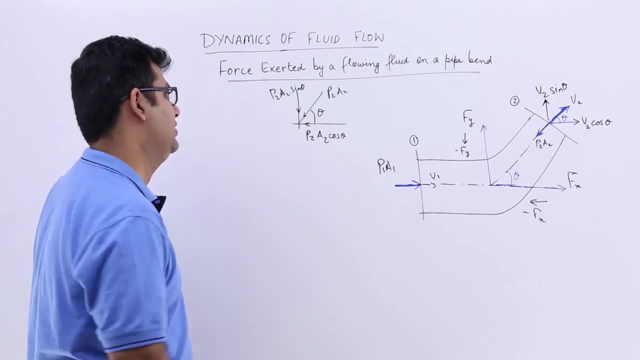 So the horizontal component would be P2 into A2 cos theta, which would be in the negative direction of x-axis, And you will have your P2 A2 sin theta, which would be in the vertically downward direction, that is, the y-axis. Okay, 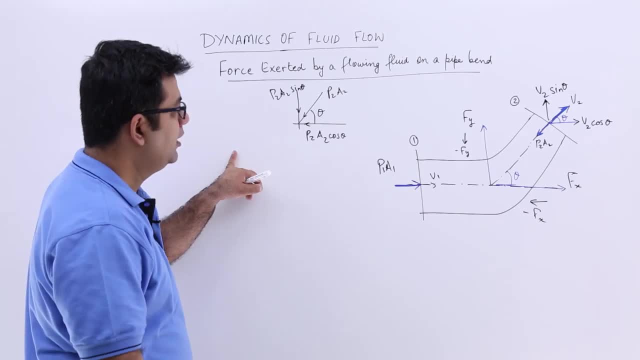 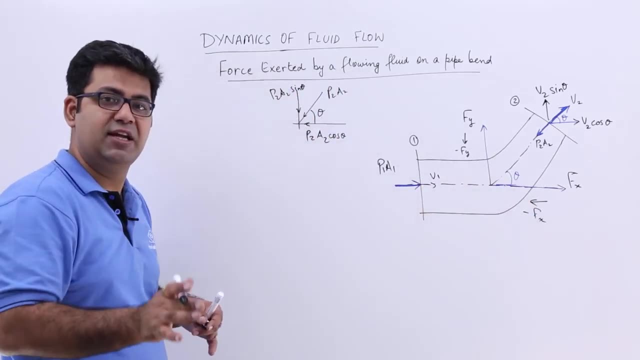 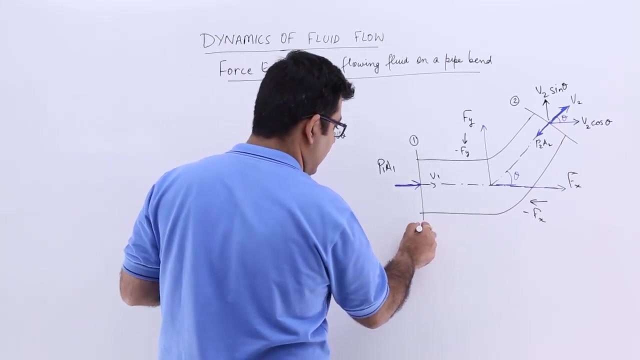 So this is what you have In terms of the forces. So now let's apply the momentum equation. The momentum equation says the net force in a particular direction is equal to the rate of change of momentum in that direction. So let us say we will take the x direction first. 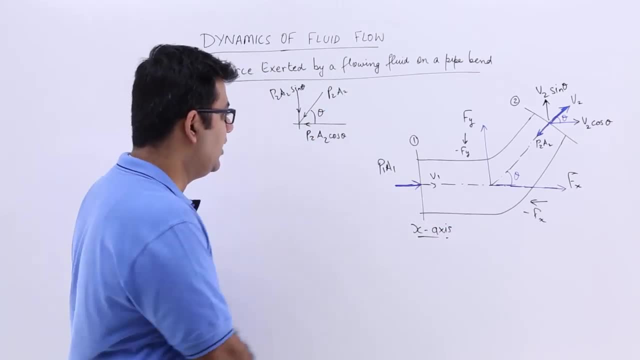 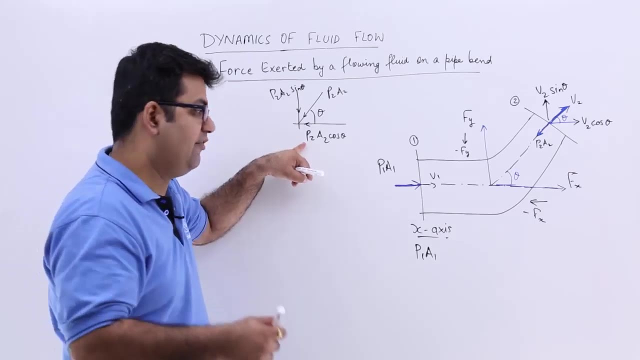 So what is the net force in the x-axis? So you will have P1 A1, which is in the positive direction. Then you have minus P2 A2 in the negative of x direction. So you will have minus P2 A2. cos theta. 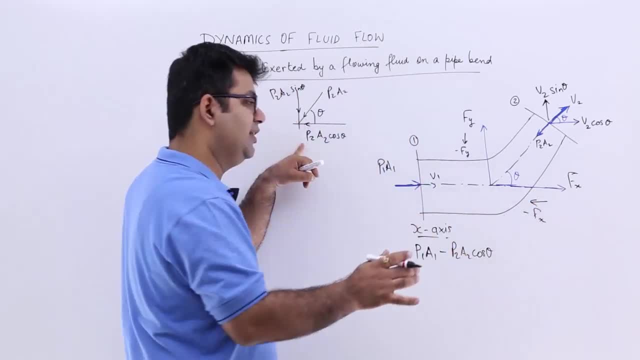 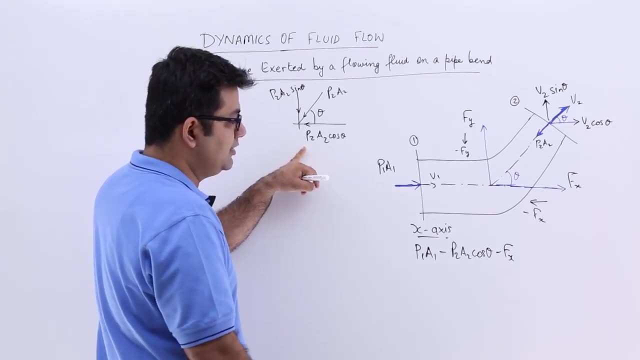 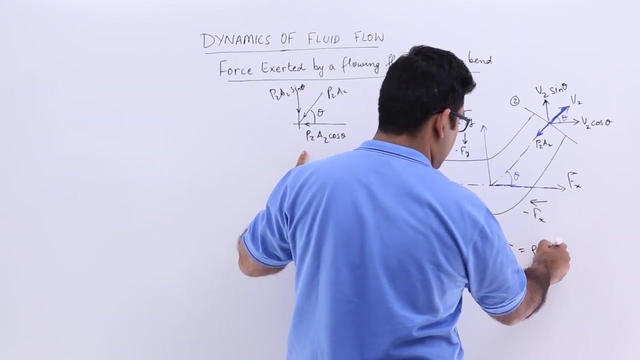 Okay, Then we have minus fx. We will always take the reactive forces, So you will have minus of fx again in the negative direction, And then this is the net force And this is equal to the rate of change of momentum. So you will be having rho into q, that is the mass flow rate per unit time, into the change in velocity. 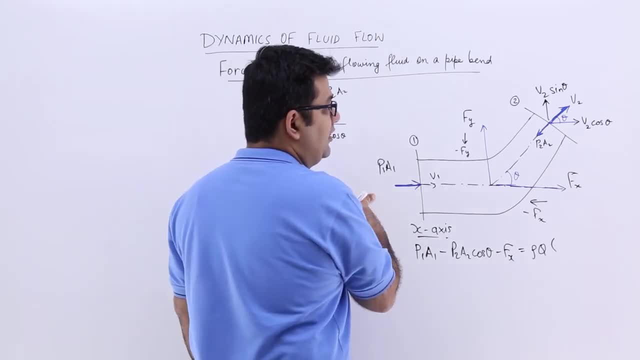 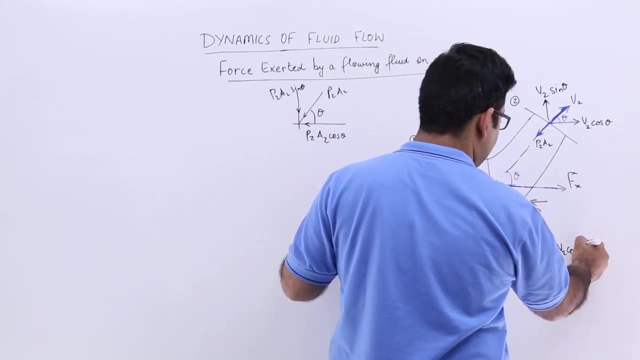 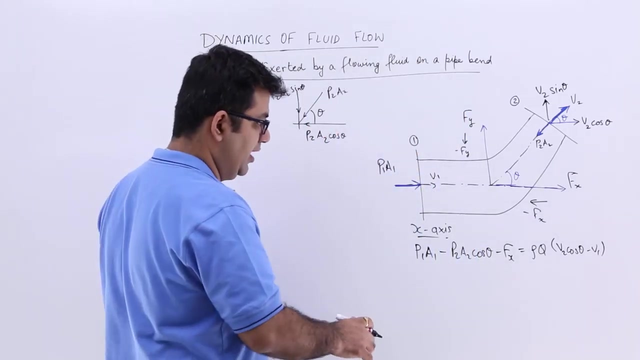 So the initial velocity is v1 and the final velocity is v2 cos theta. So change would be v2 cos theta minus v1.. That is final minus initial. So this would be your equation. So from here we have to find out fx. 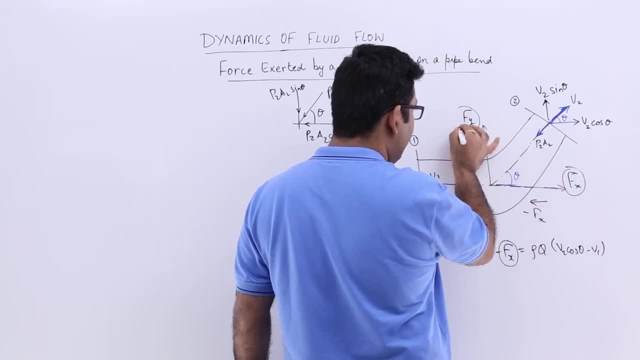 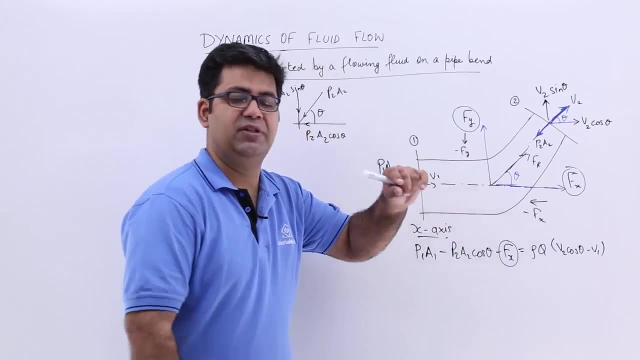 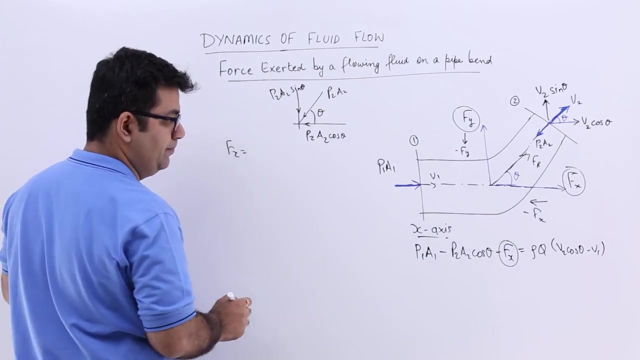 Because once we find out fx and then we find out fy, we will be able to find out the resultant force And then the angle at which this resultant force is acting. So from here, let us find out fx. So fx would be. 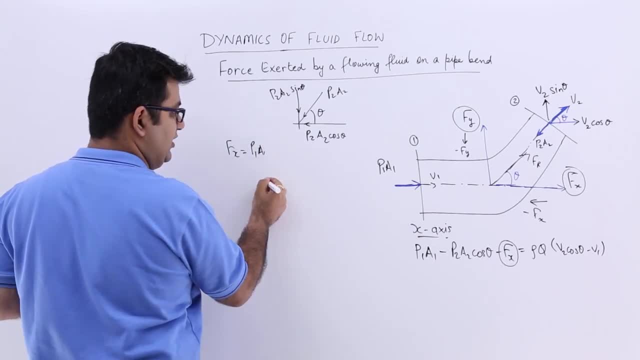 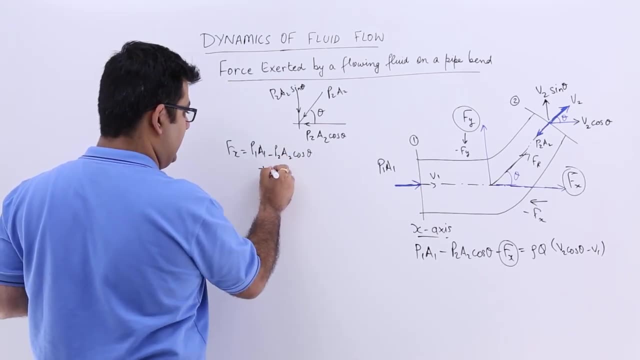 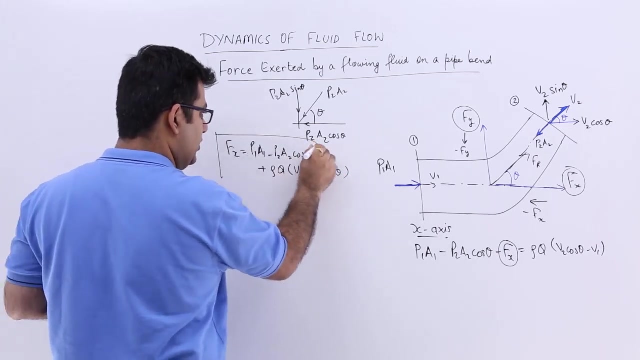 You can take it on the positive side, So you will have P1 A1 minus P2, A2 cos theta, And then it will become plus rho q v1 minus v2 cos theta. So that is the equation that I used to find out the value for force. 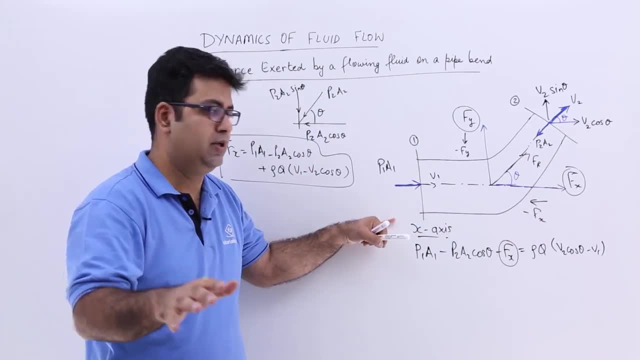 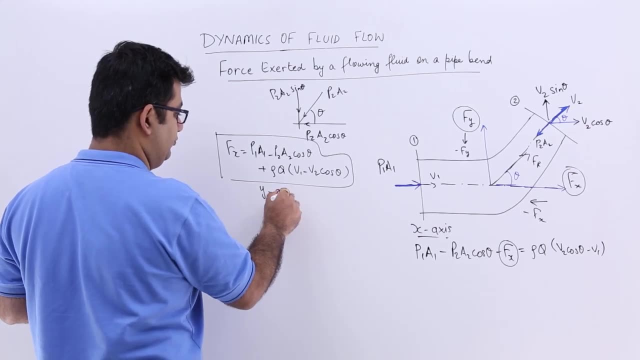 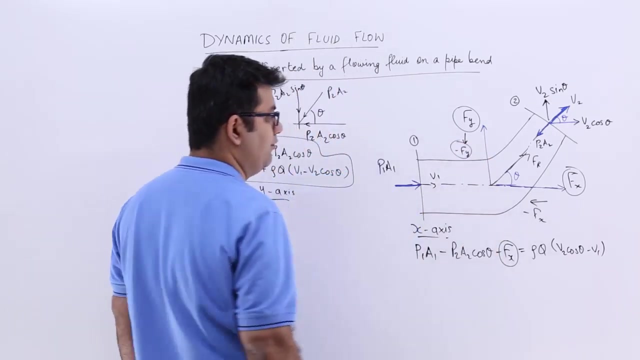 So this was the balancing of equation as per the momentum principle In the x direction. let us have now for y direction, For y axis, you have the first force as minus f of y. So there is no force, you can say from section 1.. 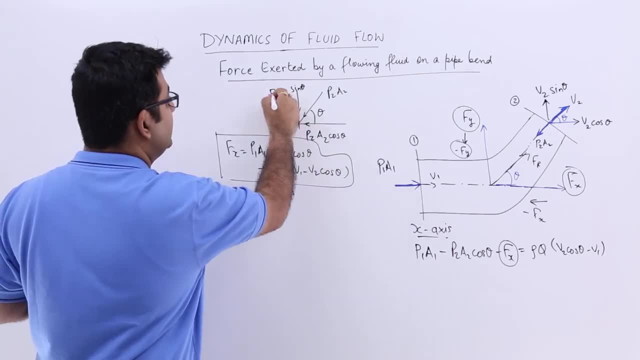 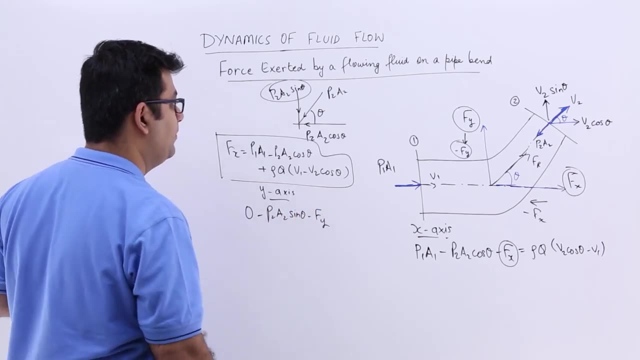 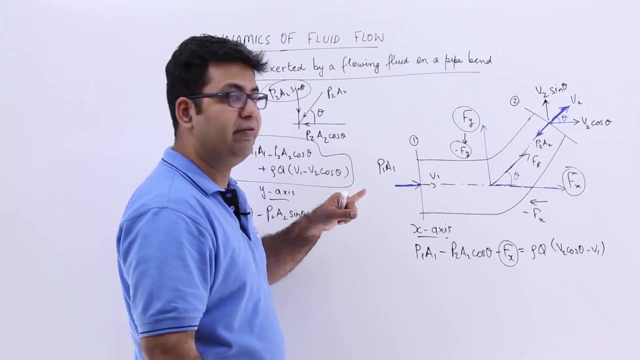 So you will have 0. in that case, Minus. you will have this Minus P2, A2 sin theta. Then we have minus f of y. This is equal to rho into q. Now, if you look at the final velocity, 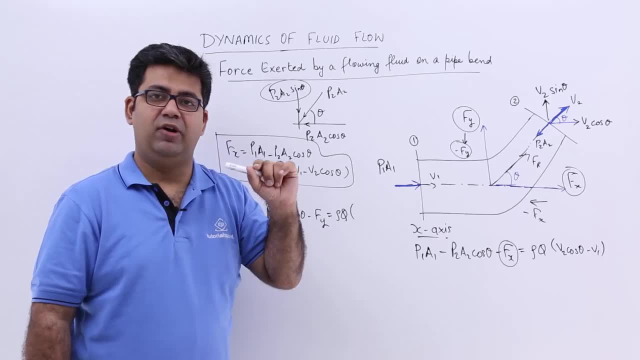 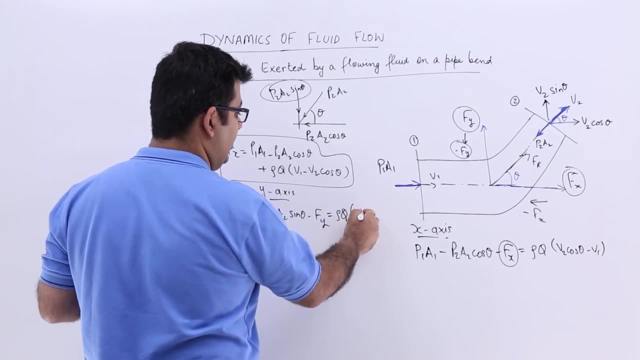 you have v2 sin theta, But there is no velocity in the initial stages in the vertical direction, So it will be 0. So you will have v2 sin theta minus 0. So from here, Let us find out the value for fy. 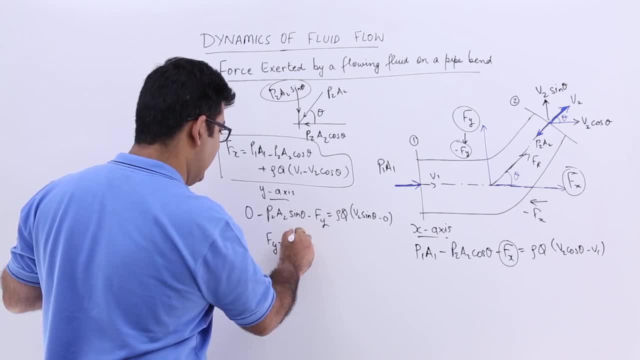 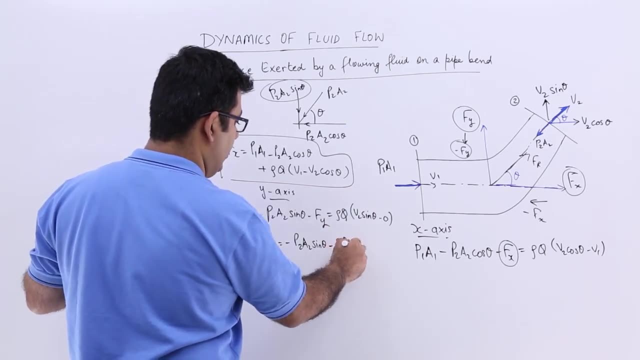 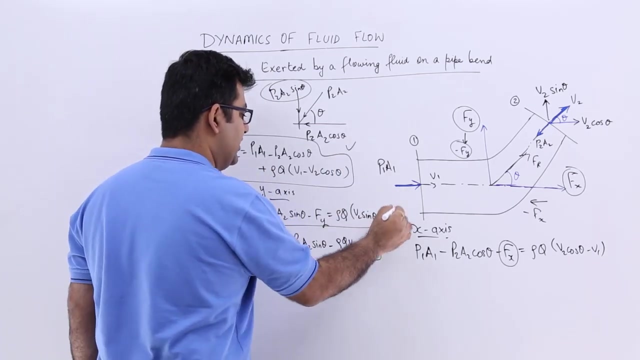 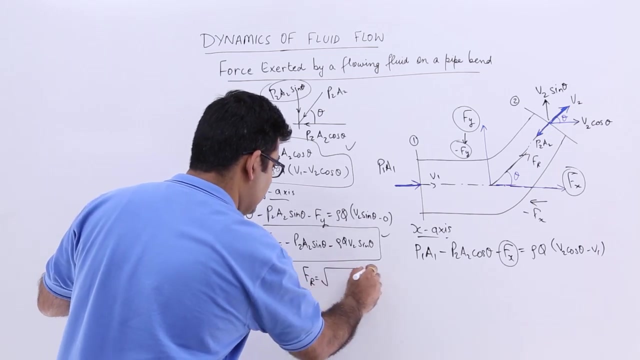 So fy would be equal to minus P2, A2 sin theta, minus rho q into v2 sin theta. So this is your fy. So now we have got fx and fy. Okay, The resultant equation, resultant force, would be fr, which is nothing but the square root of fx square. 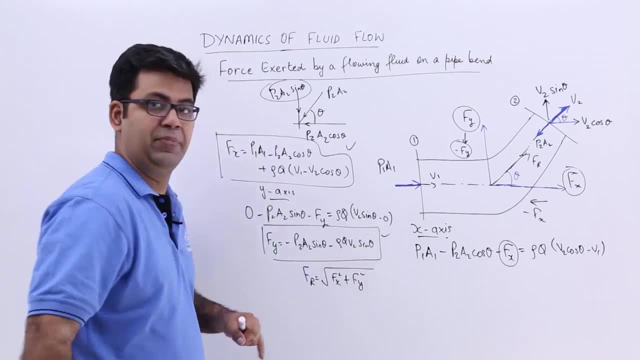 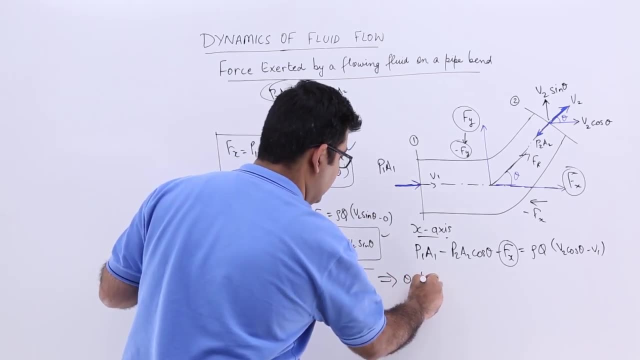 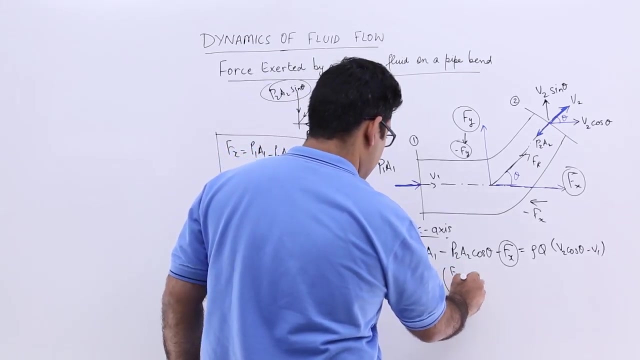 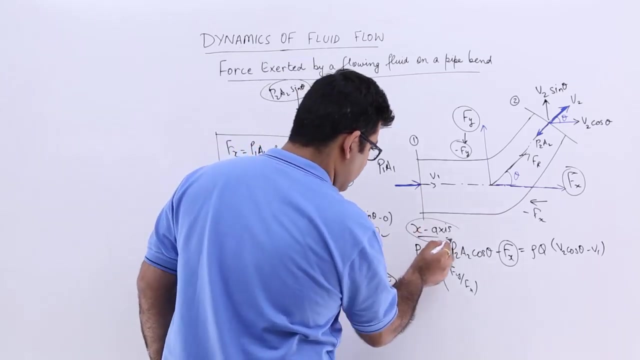 plus f2.. And from this I can easily find out the angle at which this fr is acting. So it will be theta, which is equal to tan inverse of fy upon fx, fy upon fx. So it is a very simple case. You only have to resolve forces in the direction x and direction y as per the momentum principle. 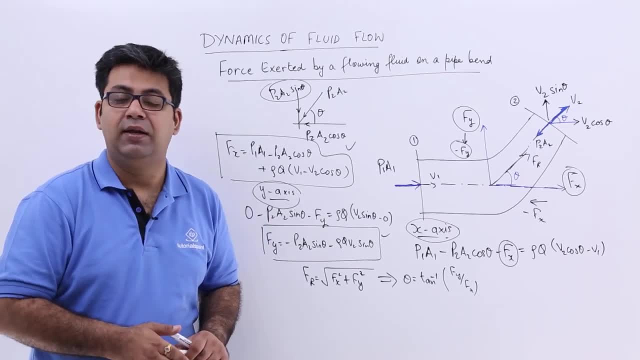 So this is all that you have to understand In the theoretical part. Now let us look at some questions on this concept. 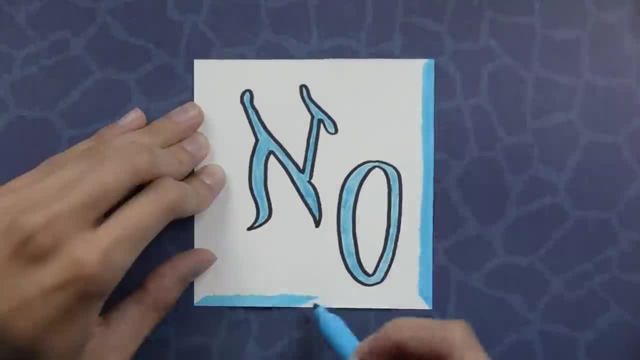 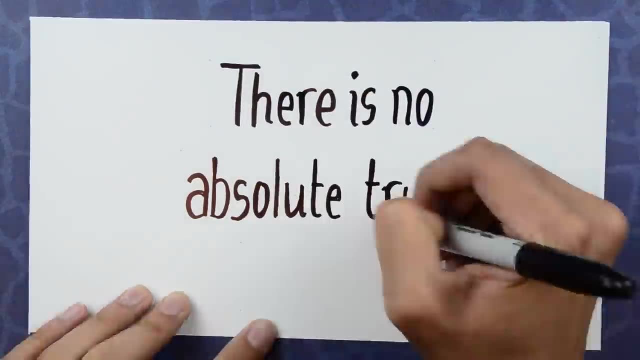 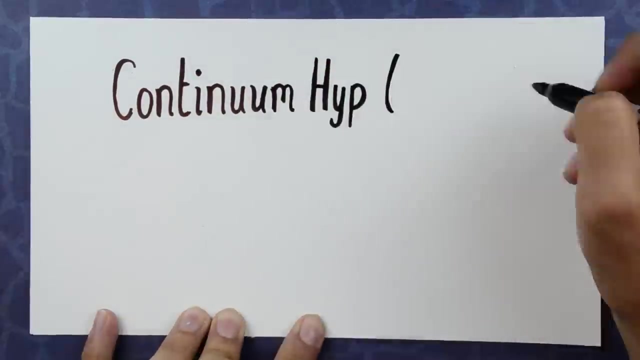 There is no absolute truth in math. Math is self-referential, so it can only prove statements about itself. This wasn't a huge problem until something called the Continuum Hypothesis appeared on the scene. Whatever this problem was, a group of people expected it to be true. 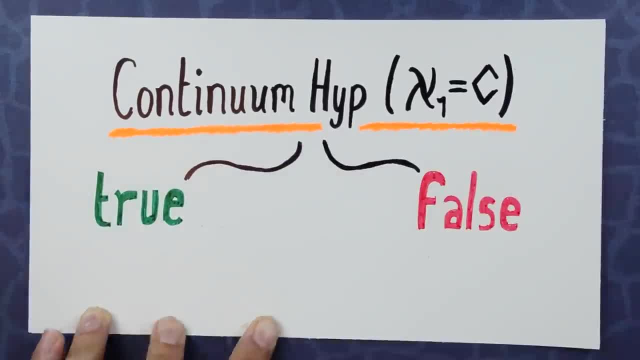 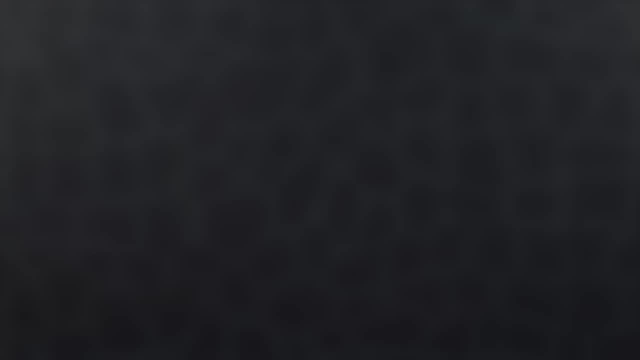 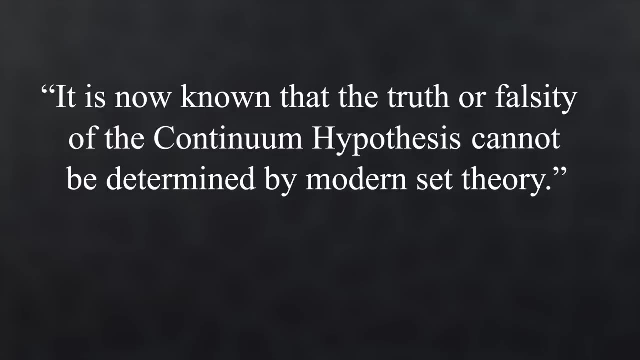 and another group expected it to be false Until it was proven that you actually can't prove that it's true or false purely from the fundamental axioms of math. Mathematician Paul Cohen wrote: it is now known that the truth or falsity of the Continuum Hypothesis cannot be decided from 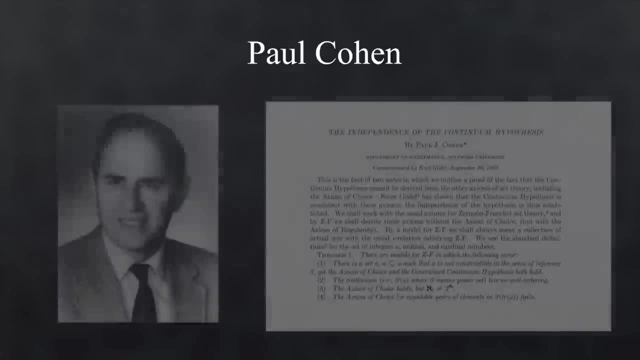 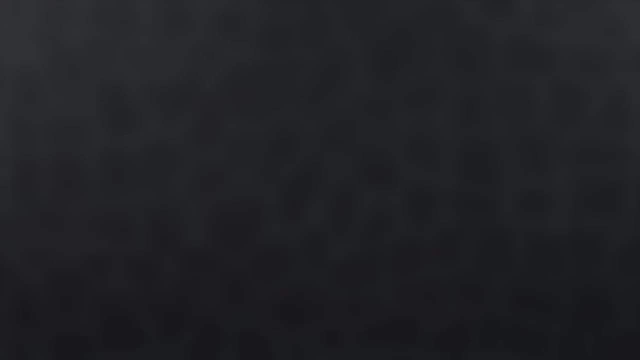 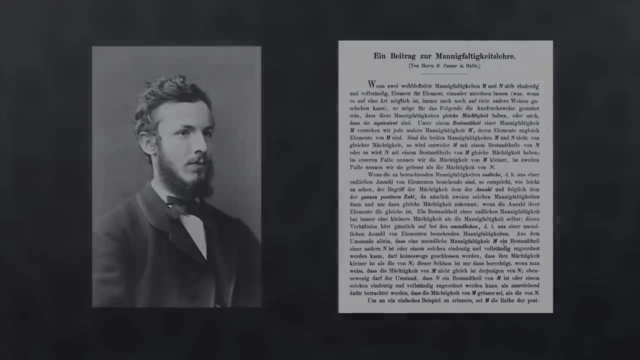 modern set theory. The same Paul Cohen won the Fields Medal in 1966 because of his contribution in proving that the Continuum Hypothesis is undecidable. But it's a little unfair if I don't at least hint at what the Continuum Hypothesis is, The person to keep in mind here. 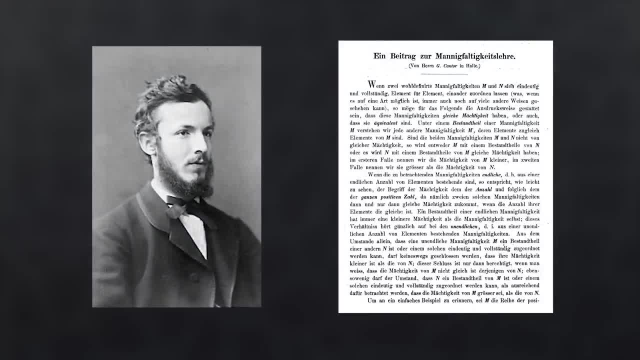 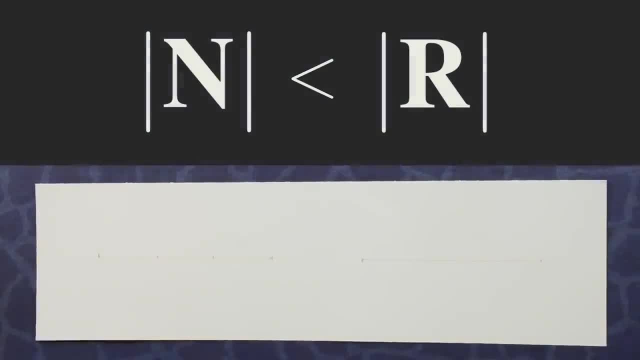 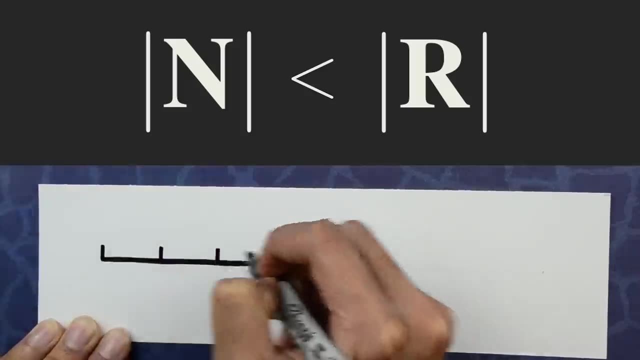 is Georg Cantor who showed that some infinite sets are in some sense larger than other infinite sets. In particular, Cantor showed that the size of the real numbers is bigger than that of the natural numbers. Intuitively, this means that the natural numbers are discrete. you can count them. 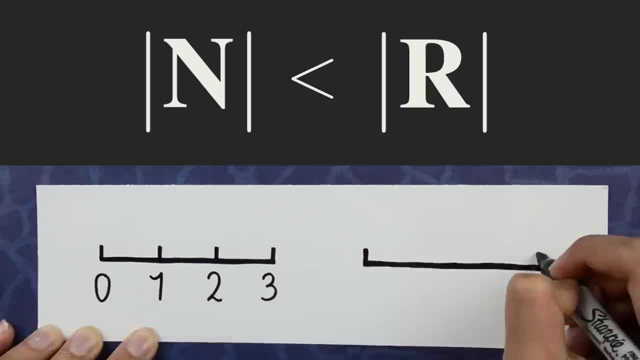 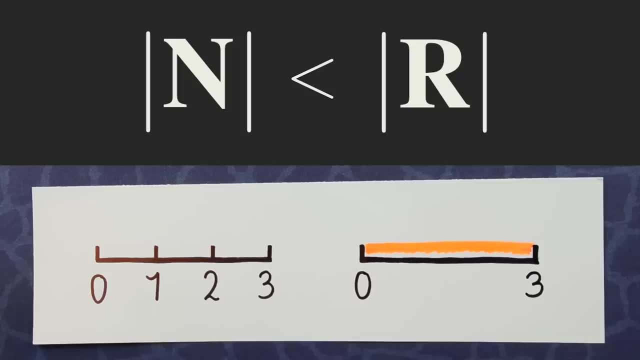 one by one. But the real numbers are a continuum. you cannot count them one by one. So it's plausible that in some sense there are more real numbers than natural numbers. Cantor asked a very simple question: Is there a set X whose size is in between these two?